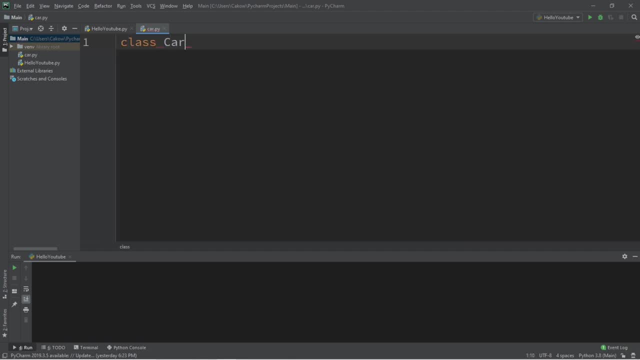 our class within the separate module, So class car, and for now I'll type in pass. Then we just need to import this class. So within our main module we would type from the name of the module: import the name of the class. 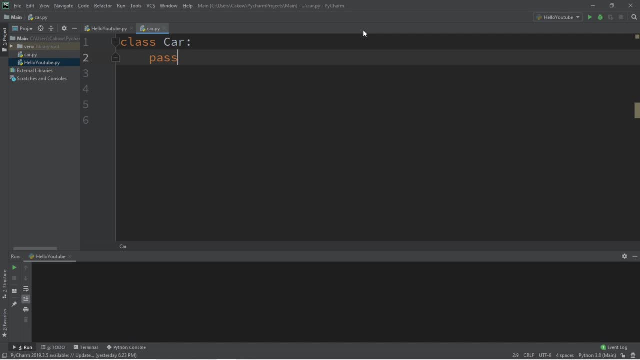 From car import car. Now, objects can have some combination of attributes and methods. Attributes describe what an object is or has. So what are a few attributes that cars might have? They might have a make, so let's create a few variables. 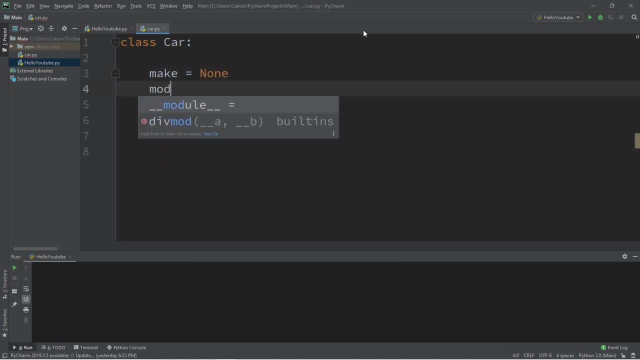 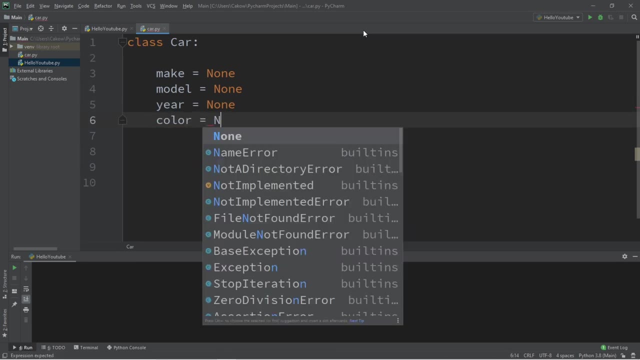 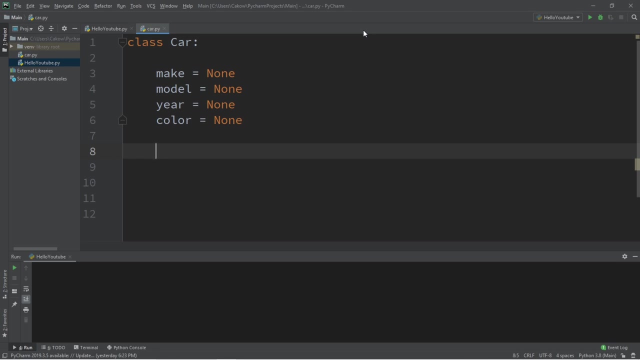 For the time being, I'm just going to use none because I play this. older Cars can have a model, a year and a color. Now, objects can also have methods. What kinds of methods could cars perform? Perhaps a drive method and a stop method? 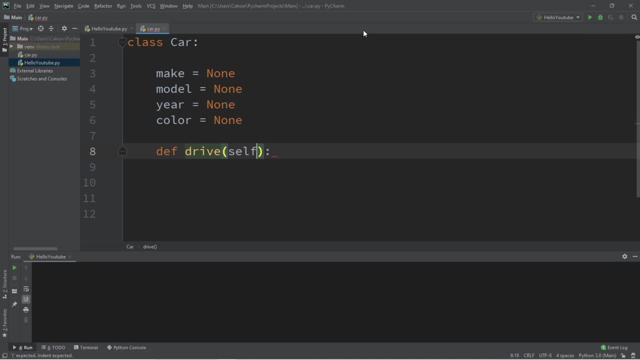 So let's define those Def. let's say drive, and we'll have one argument: self Self refers to the object that is using this method. Now, what do we want to do when we call this method? Let's say this: 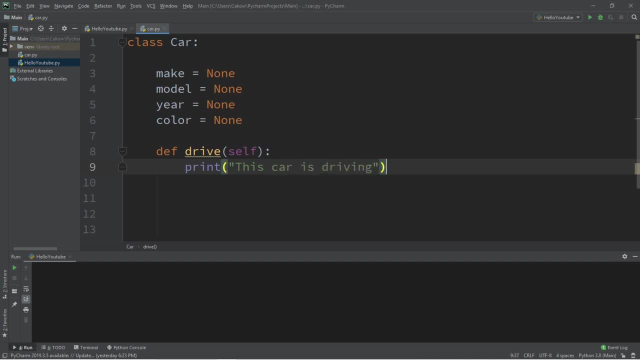 car is driving. Let's create a stop method as well: Def stop, and we will print this car is stopped. We now have all of the different attributes and methods we would like our car objects to have, but there is one more thing that we need. 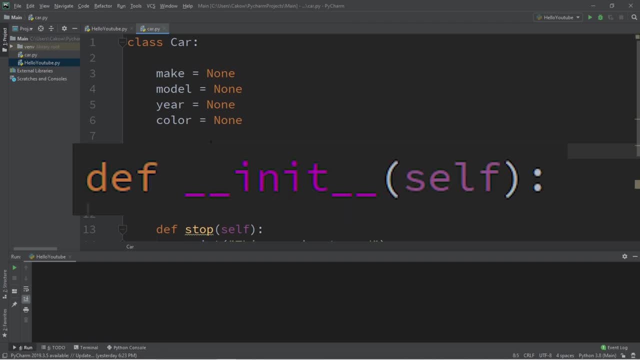 It is a special method called the init method that will construct objects for us. In other programming languages this is known as the constructor. So we need a special method that will create objects for us. So we need to define this method. def. 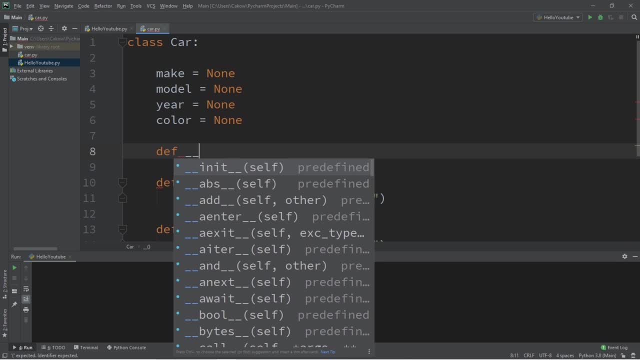 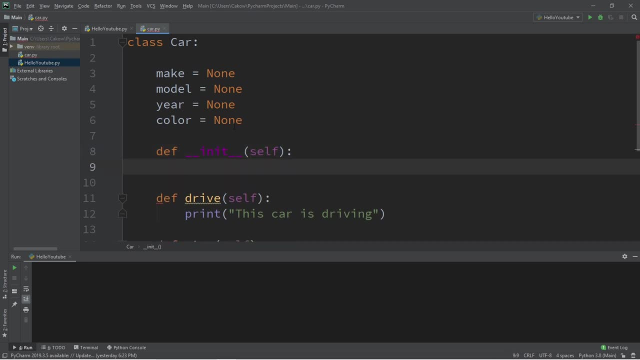 and the syntax on this is somewhat strange. It is two underscores, I-N-I-T It's short for initialize two underscores again, and then we need at least self as an argument, And then we can actually assign our car objects unique variables. 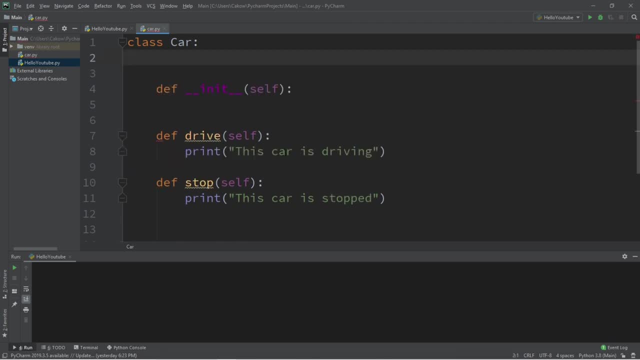 So take all of these attributes that we have and we're going to place them within this init method. Now we can receive arguments when we create car objects, but we need to pass them in as arguments for our car objects, So we need to set up some parameters. 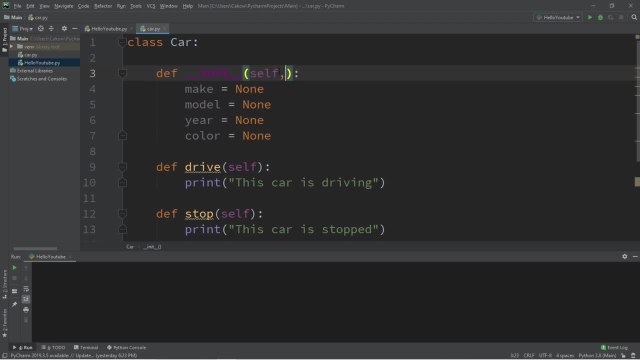 Let's say, in order to create a car object, we need a make, a model, a year and a color. Then, when we receive these arguments, we can actually assign them to each car's specific attributes. But we need to precede each of these with self. 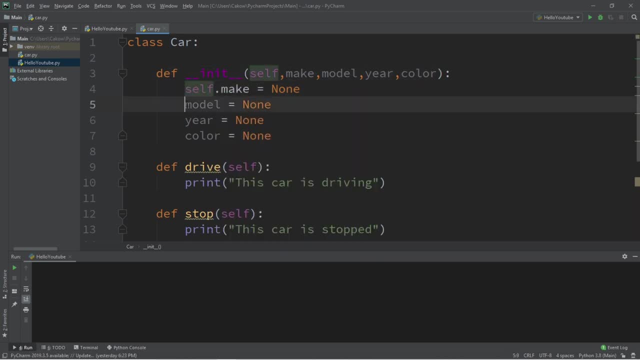 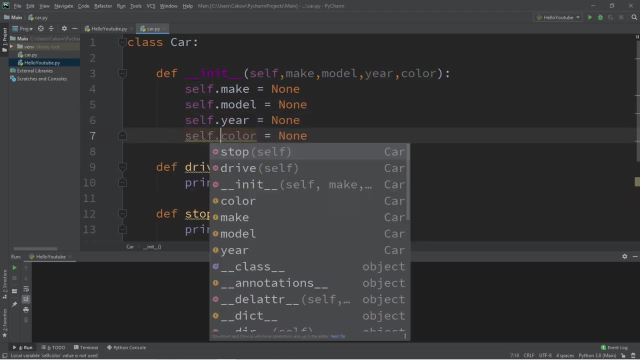 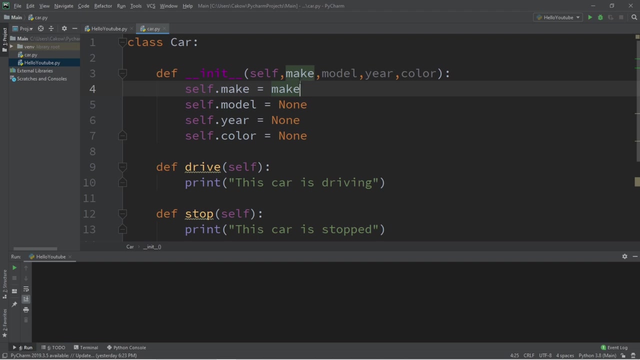 Self is referring to the object that we're currently working on or creating. So selfmake, selfmodel, selfyear and selfcolor. And then when we assign these, we're going to say: selfmake equals whatever make that we receive when it's passed in. 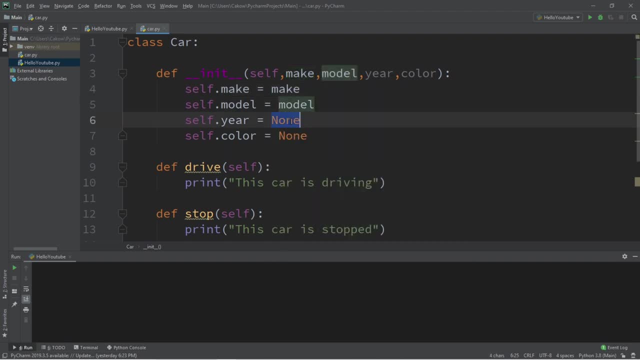 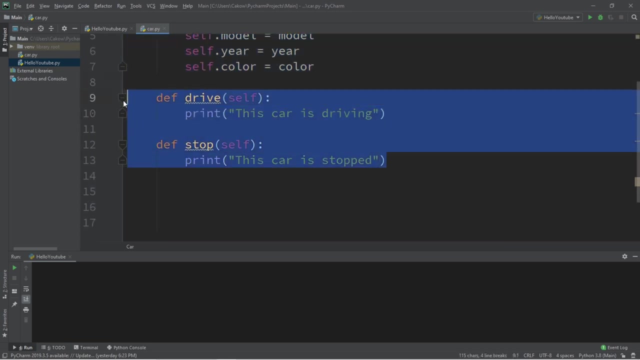 as an argument. Selfmodel equals model and continue that pattern for year and color. Alright, that is all we need for our class car. We have a constructor, we're assigning arguments that we receive to the attributes of our car object and we also have two methods. 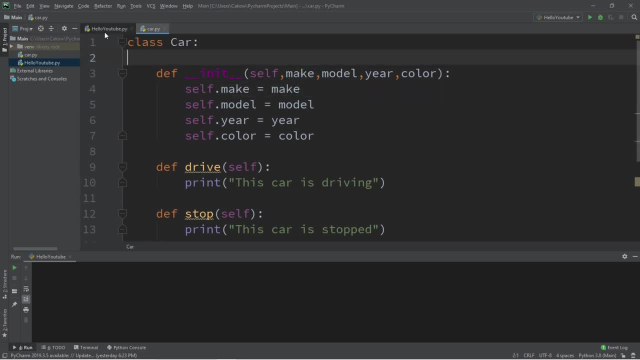 one for drive and one for stop. Now we can start creating some car objects. so, going back to my main file here, to create an object we need a unique name for it. Let's call this first car just. car1 equals the name of the class. 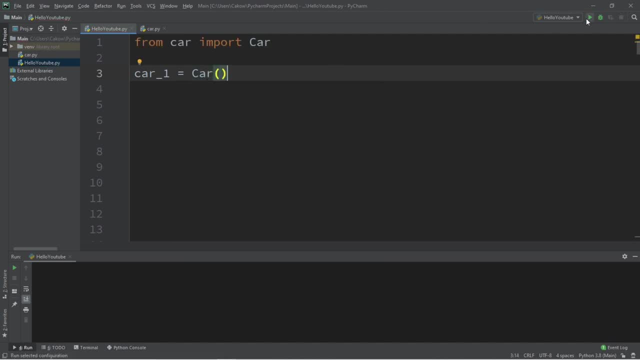 car, then a set of parentheses. Now, in order to construct a car object, we need to pass in a matching set of arguments. You can see here that we need to pass in a make, a model, a year and a color. 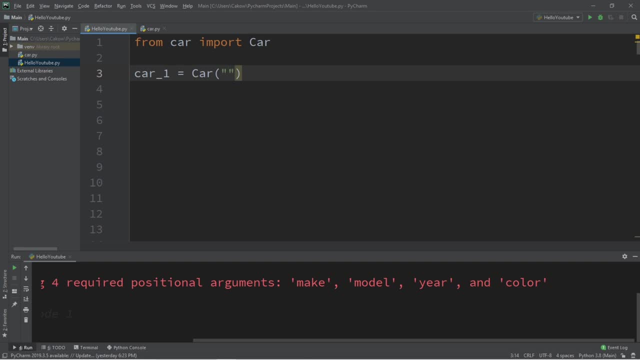 So what kind of car should we make? Let's say that the make is going to be Chevy. We need a model, perhaps Corvette. a year 2021 is good, and a color, let's say blue. Alright, now let's actually access. 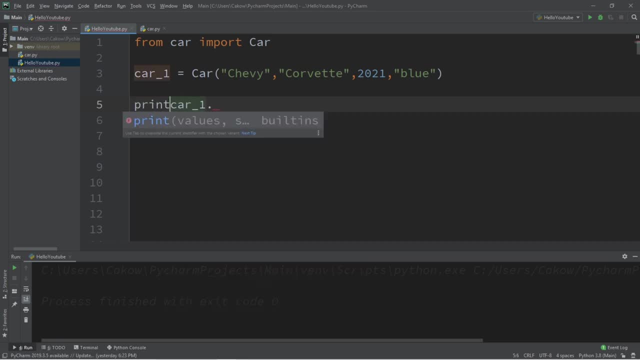 some of these cars' attributes and I should probably put this within a print statement. So print car1's make and this should print Chevy. Then we can do the same thing for model year and color. So let's change some of these around. 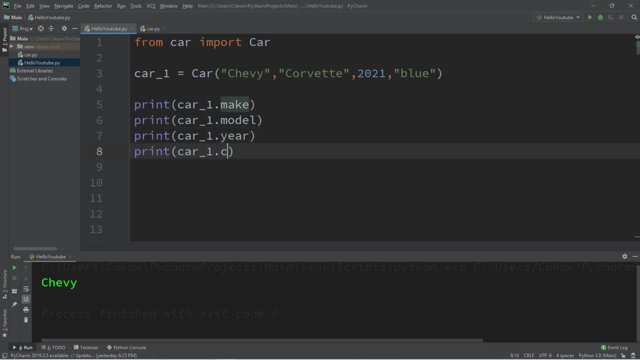 Model year and color: Yep. this object is a Chevy Corvette 2021, and the color is blue, And we should have two methods as well. So, car1,, I would like this car to use its drive method. This car is driving. 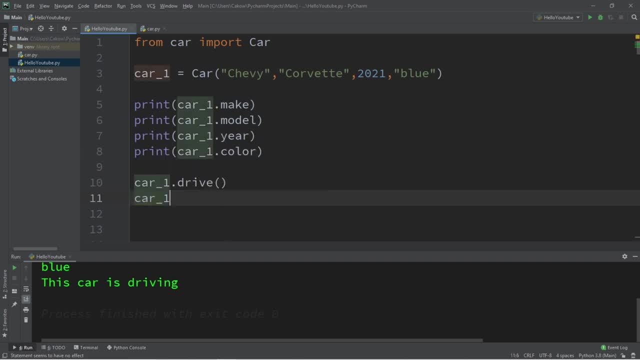 And let's have this car use its stop method- car1.stop- This car is stopped. There's one thing that I should mention real quick, because I forgot to mention it earlier. So within our init method, you can see that we need five arguments. 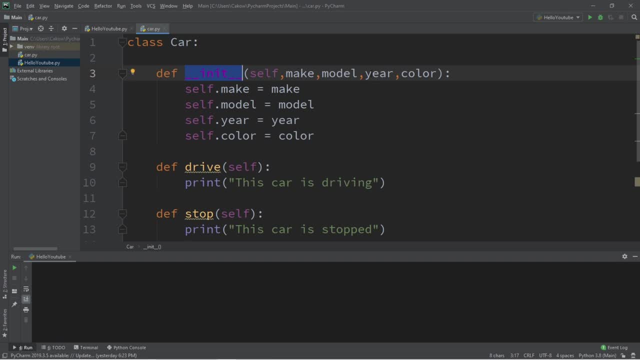 in order to construct a car object, self make model year and color. But when we pass in our arguments we're not passing in anything for self. We only have four arguments here. That's because with Python we do not need to pass. 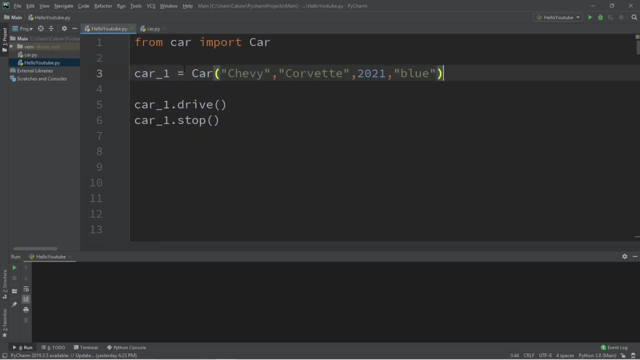 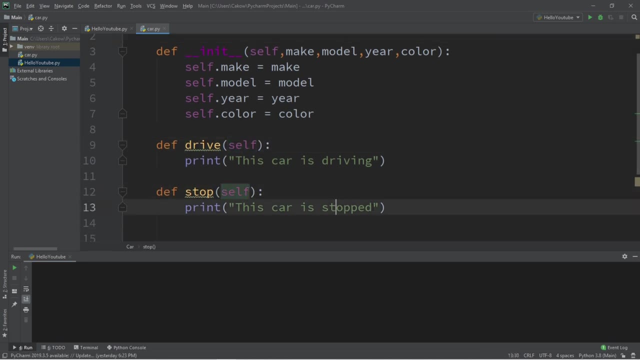 in self. That's done automatically for us. We're referring to the object that we're dealing with. As you can see, with our drive and stop method we need to pass in self in order to execute our method, But when we call this method, we do. 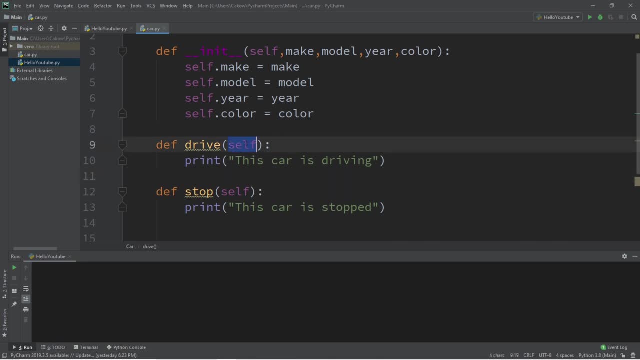 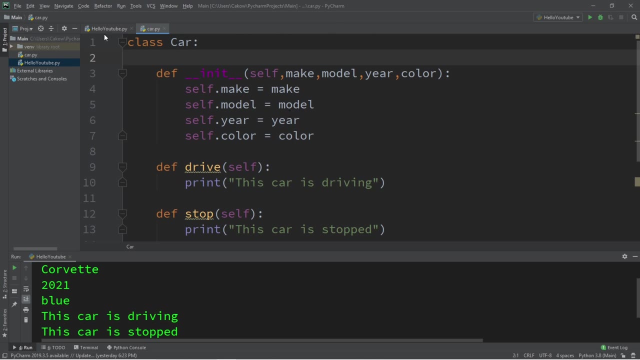 not need to do so. So just remember: with Python with self, we do not need to pass in anything for this argument. That is all Now. the nice thing about this is that we can reuse this class as a blueprint to create more car. 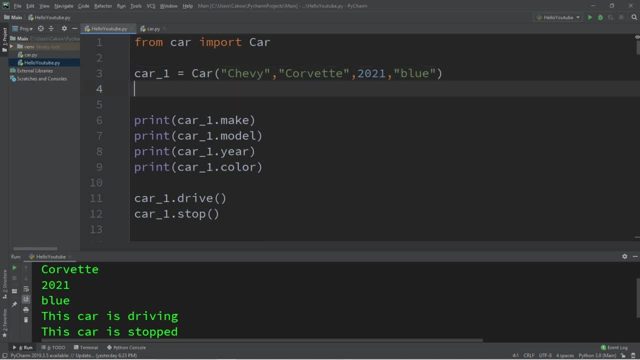 objects. We just call that init method, that constructor. So this time let's create a second car called car2.. And this will be a different kind of car. What kinds of arguments should we pass in? Let's say, this is a Ford. 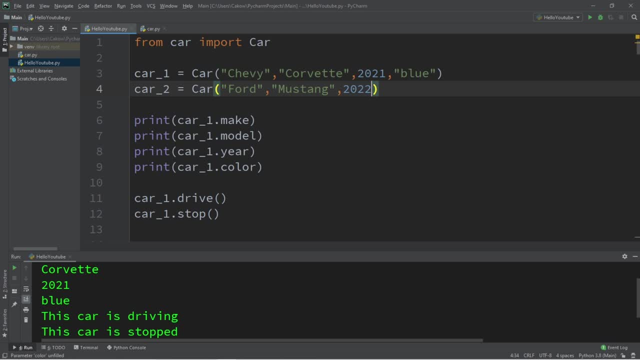 Mustang, The year will be 2022, and the color will be red. Alright, let's check car2's attributes And let's have car2 use its drive and stop method. This is a Ford Mustang. The year is 2022.. The color is red. 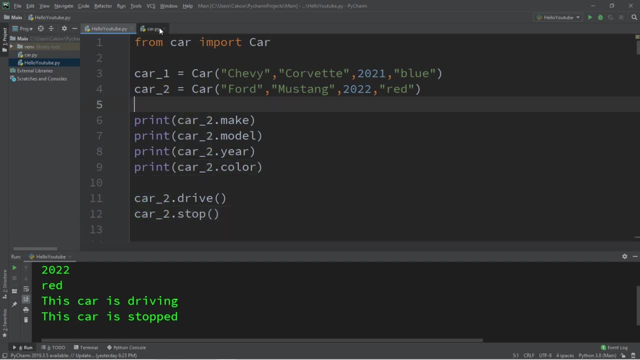 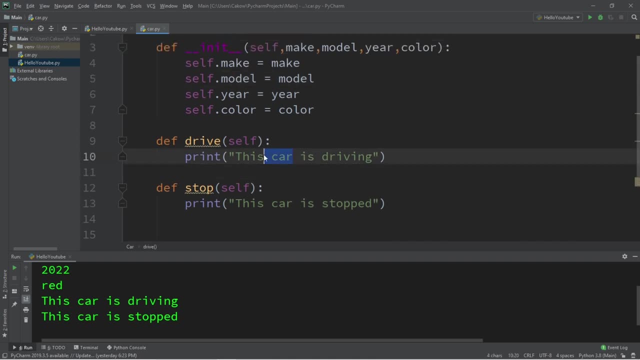 This car is driving and this car is stopped. One other thing that we can do, too, is that, within our methods here, let's replace car with the name of the model that we're working with. So this plus self dot model plus is driving Now this: 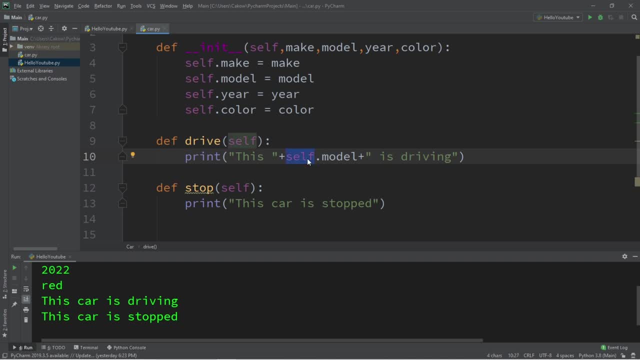 self keyword. think of it as you're replacing self with the name of the object that we're working on. If car1 is using its drive method, replace self with car1.. If this is car2 that called this method, then replace self with car2..